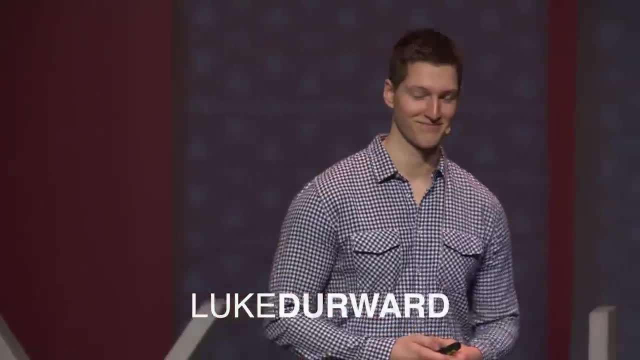 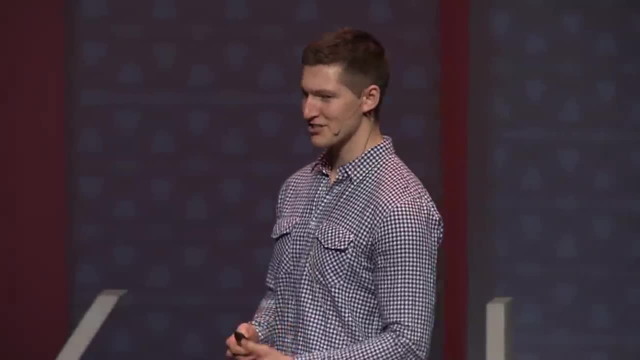 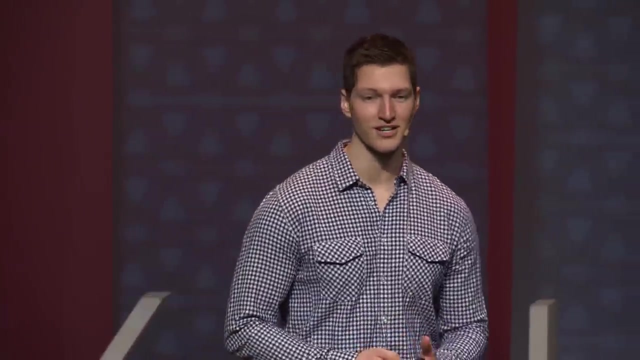 He got all excited because he thought I said poutine. The second thing he was good at was eating large quantities of food Come dinner time. it wasn't uncommon for him to out-eat most of the adults at the table. Now, as you may have guessed, as a five-foot-nothing little boy. 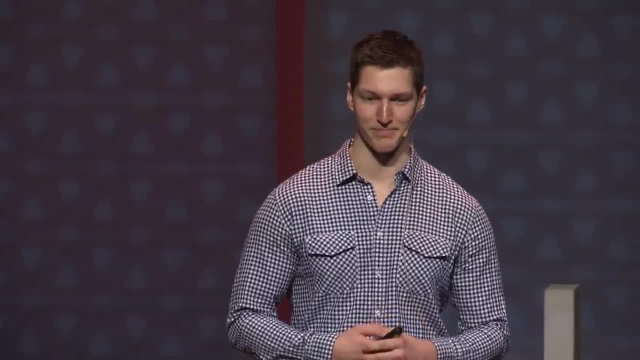 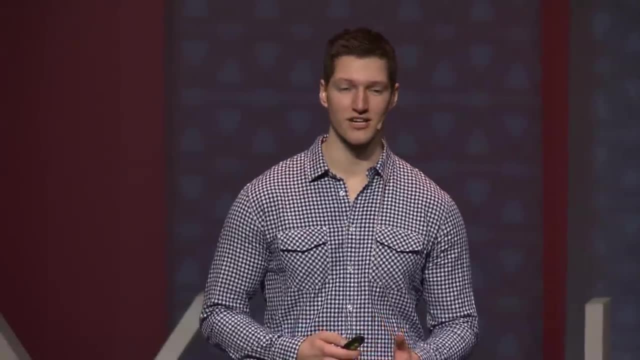 there is, in fact, a downside to regularly out-eating full-grown men. At just 11 years old, I could already see that, if nothing else changed, my little brother was headed for an adolescent life littered with teasing and unhealthy eating. As his older brother, I wanted to do something about it. 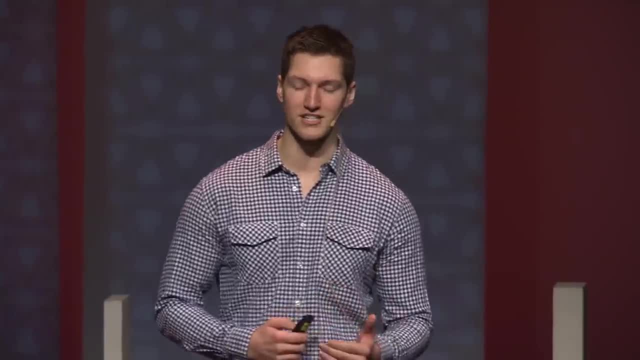 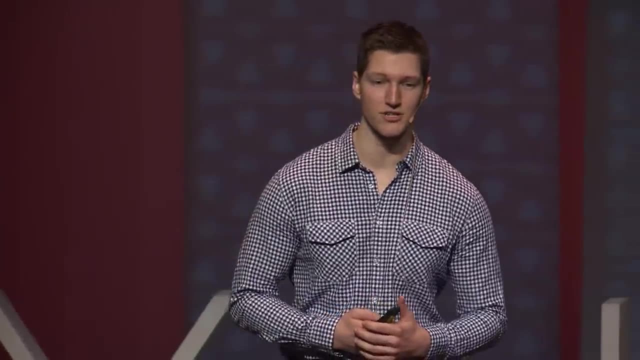 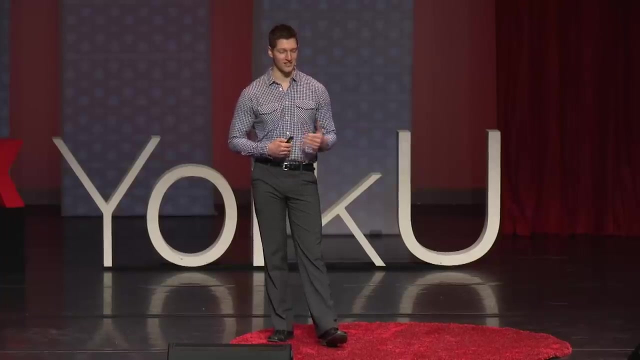 As a nutrition or a kinesiology student with an intense interest in nutrition, I knew that I had to do something about it. Initially, I wasn't sure how, but I was determined to find a way. Now, in March of 2013,, I broke my leg while I was walking to class and I slipped on some ice. 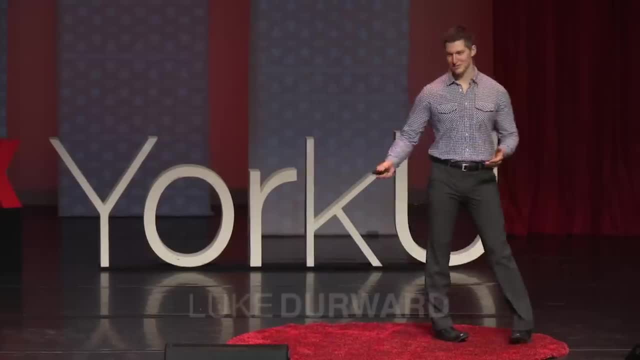 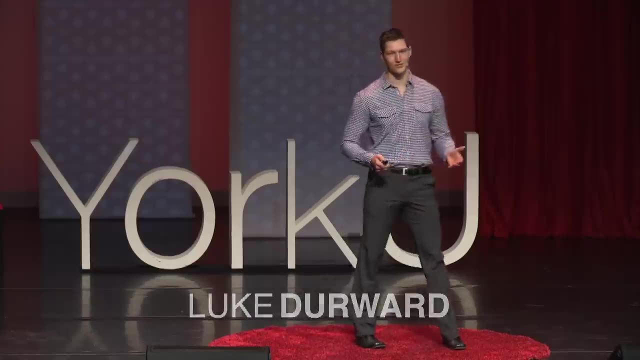 Yes, that is a lie. Yes, that is a lie. That is the whole story. I was walking, there was some ice poof, broken leg, No lives saved, no purses returned, no cool story to tell. Well, little did I know as I laid there in that quickly melting puddle of ice. 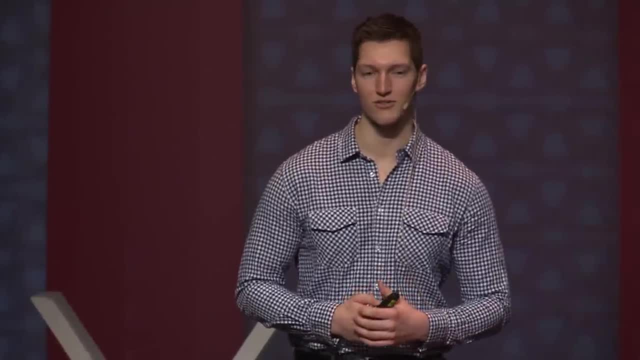 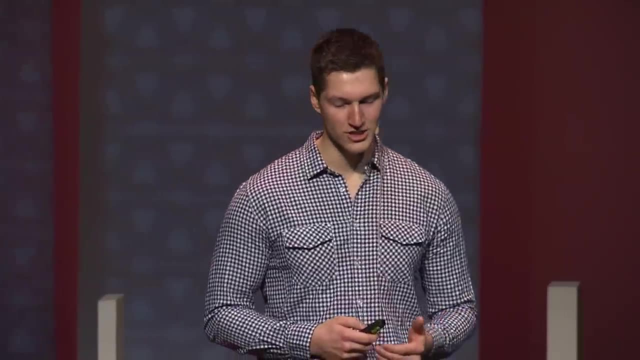 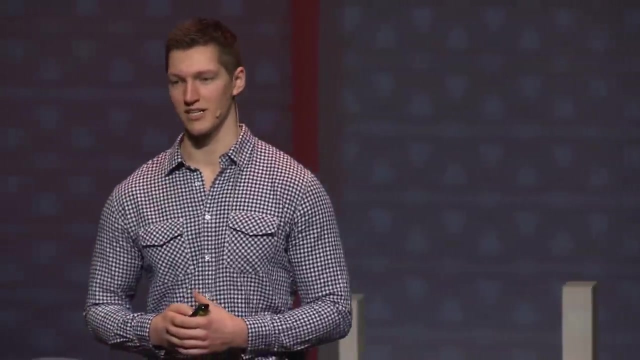 waiting for the ambulance to arrive, that this moment would forever change the life of my little brother. After I had a surgery to attach a small titanium plate and a few screws onto my fibula, I was given two crutches and told not to put any weight on my leg for two months. 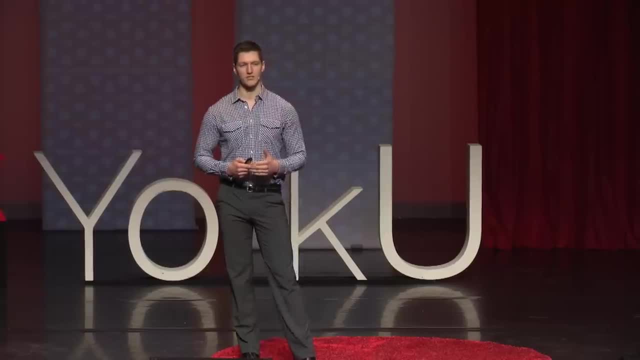 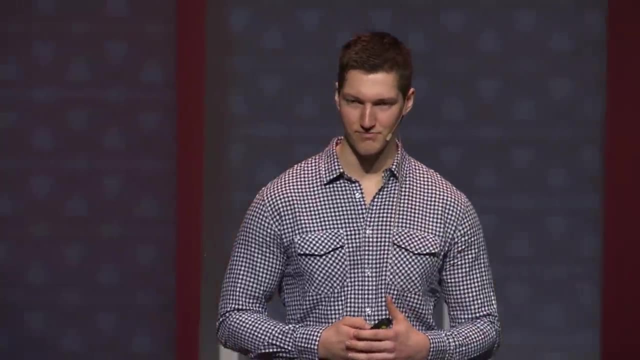 This posed a unique problem, as there was still plenty of snow and ice on the ground and I still had two months left of class, spread out over one of the largest campuses in the country. So, with that in mind, I made one of the a decision that any other hardworking student in my position would do. 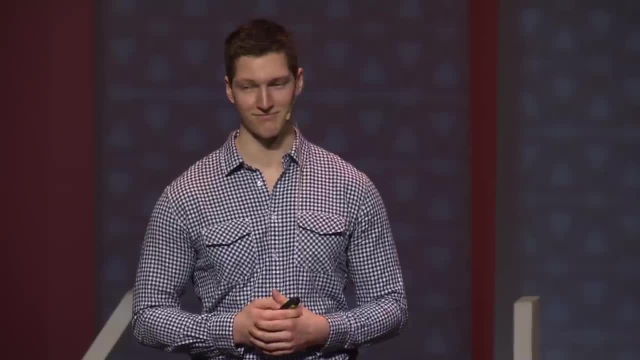 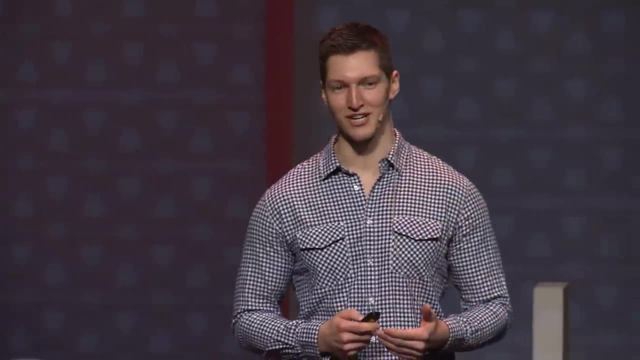 and I obviously decided to stop going to classes Now, with all this free time from studying at home. I had no idea what I was going to do. I had finally figured out how I was going to help my little brother. I knew that what he needed to do was very simple in theory, but very difficult in practice. 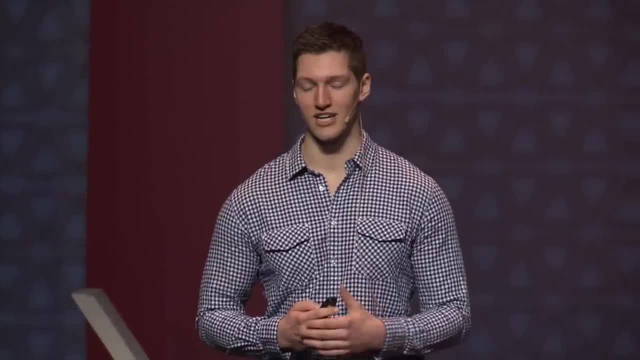 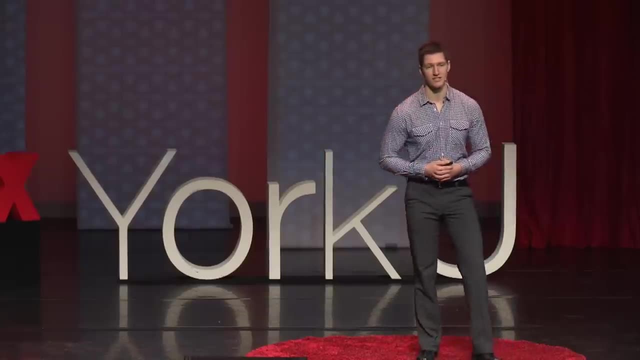 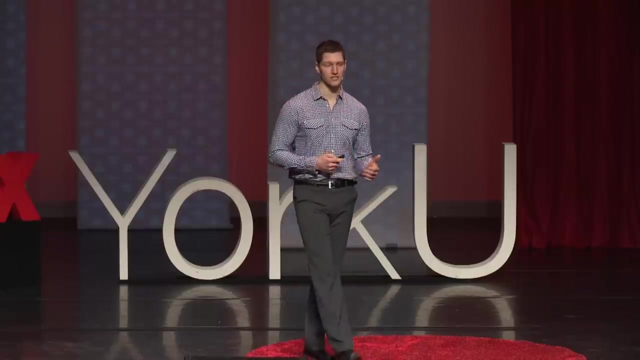 What he needed to do was change his eating habits. From experience, I knew the things that he needed to change and the things that he didn't. The problem was that communicating this through somebody else would most likely just end up like the childhood game of telephone. 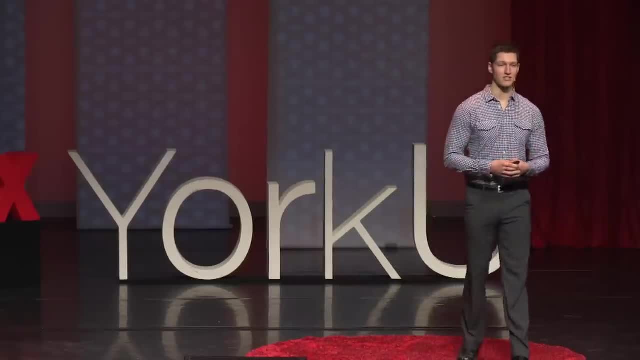 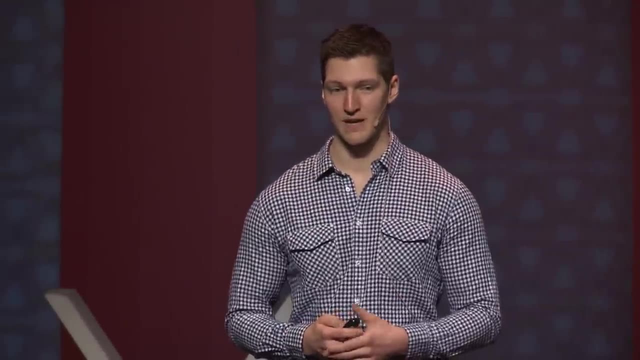 The message gets passed along, but with little misunderstandings and misinterpretations along the way. there's not much left of the original message and everybody's just left confused, And my little brother's eating habits are left unchanged. So, keeping that in mind, I made one of the best decisions of my life. 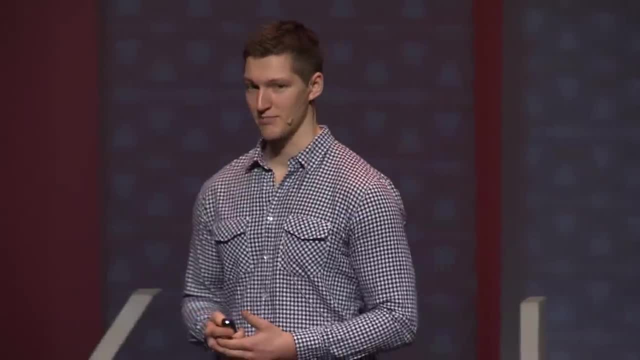 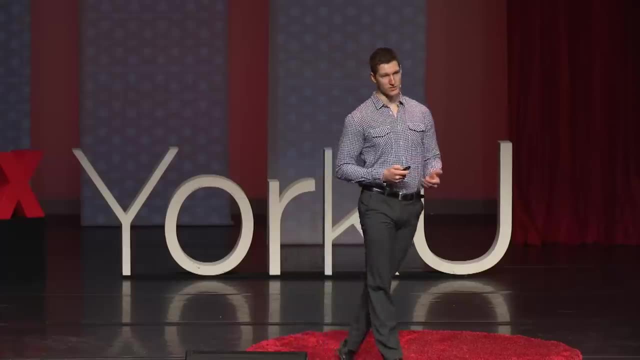 and I decided to move back home for the next two weeks and make every single meal that my little brother would eat, educating him about proper nutrition along the way. While I was at home, in the kitchen, I often found myself awkwardly trying to maneuver. 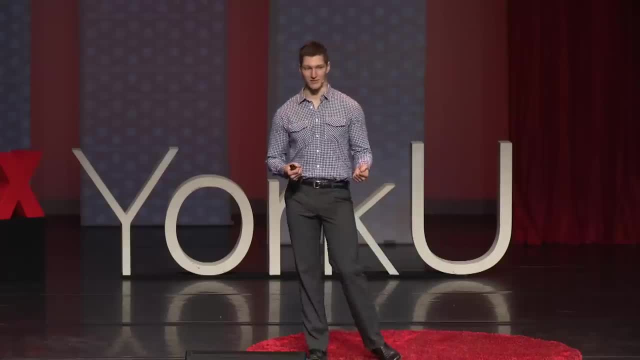 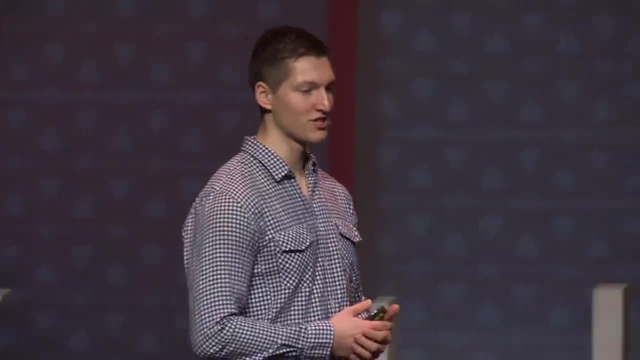 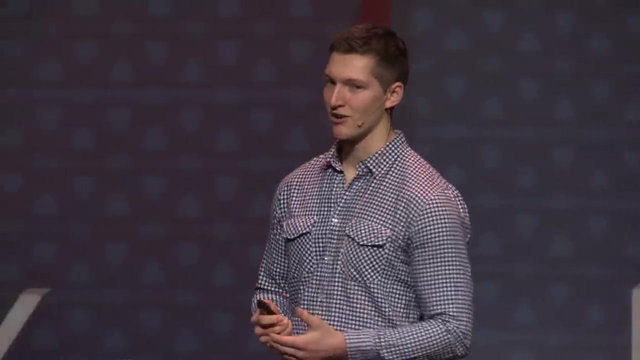 holding onto two crutches, hot pans and sharp knives. It wasn't very easy. I also had to make sure to take little breaks every few minutes to make sure that the swelling in my ankle wouldn't become unbearable. Now, after just two weeks, not only were the results phenomenal, 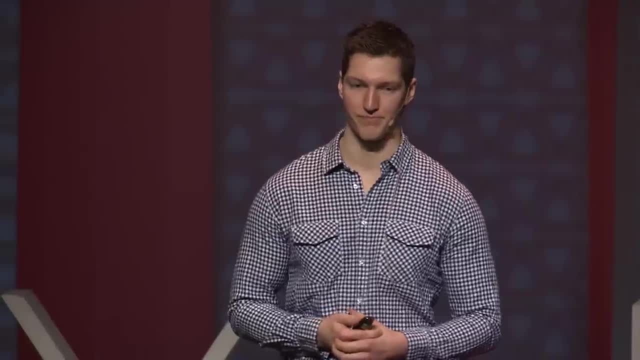 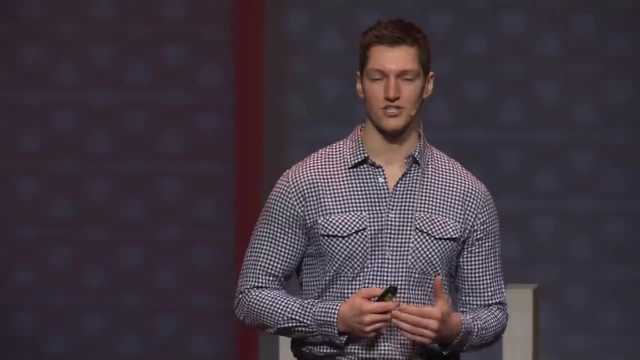 but they were as a result of a strategy that anybody can use. The reason we were able to see such dramatic and positive results, which I'm very excited to share with you later, is that we changed his environment to match his goal. We made his environment work for him instead of against him. 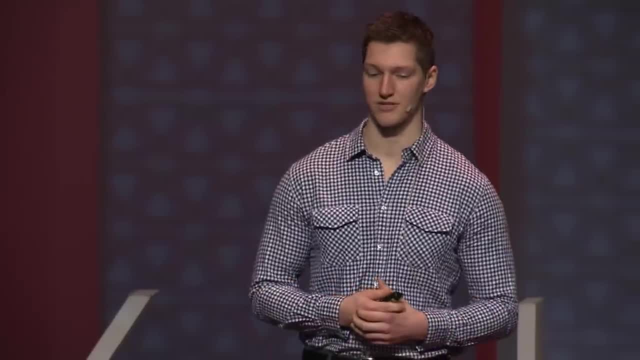 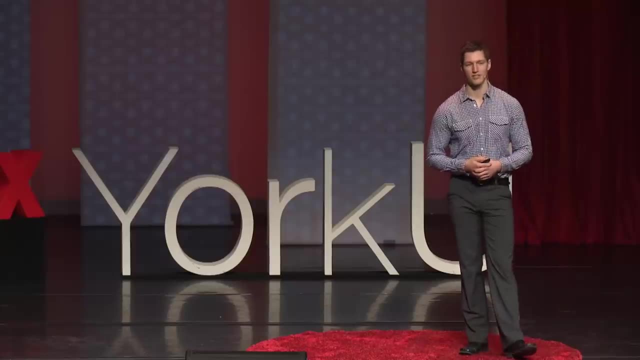 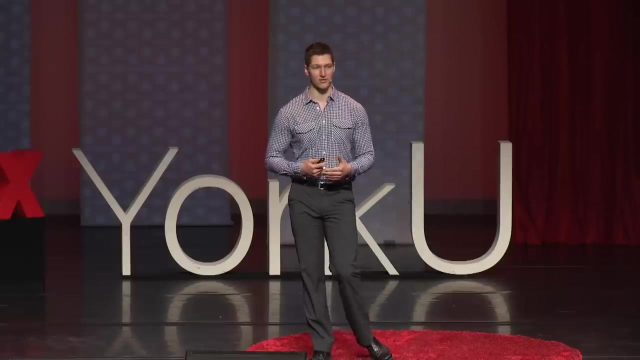 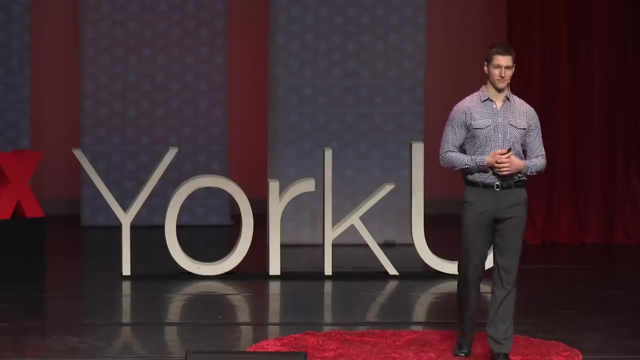 This simply meant replacing all of the bad options with healthy ones. Making this uncomplicated adjustment enabled us to easily transform his nutrition from the standard American diet, ironically referred to from its acronym SAD, to wholesome and nutritious, without a hitch. Because of the planning, this wasn't the least bit difficult to do. When you remove the unhealthy options, wholesome and nutritious food becomes both plan A and plan B. The beauty of this solution is that it takes willpower almost completely out of the equation. Quite simply, if it's not there, you can't eat it. 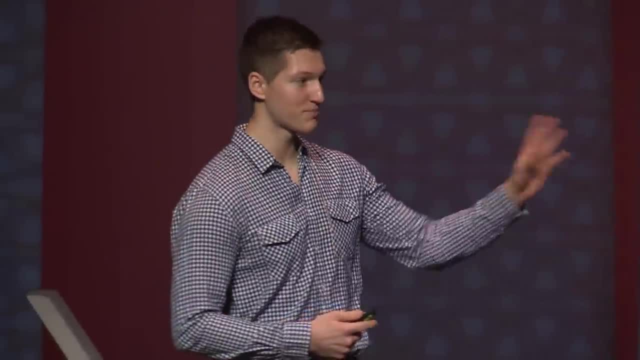 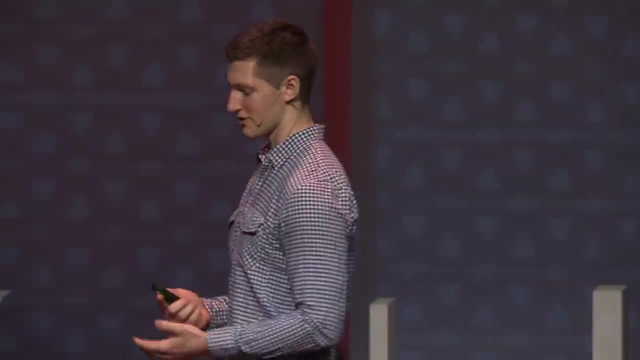 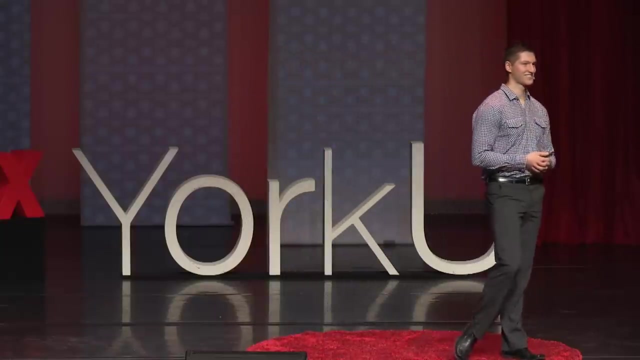 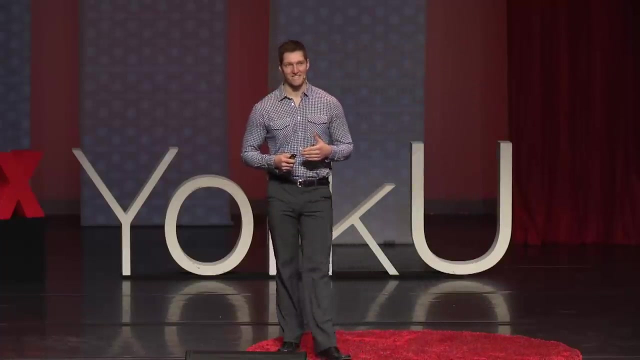 An added bonus to this strategy is that if there's no chips on the counter calling your name, it's likely that you'll just forget about them and completely avoid the feeling of deprivation all at once. A little bit of a brain block. This may sound a little bit too simple to be true, but I assure you it's not. 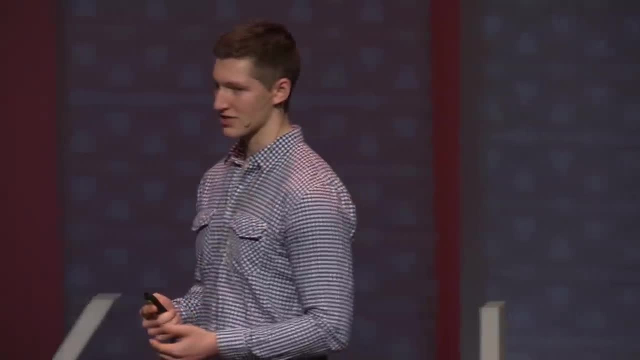 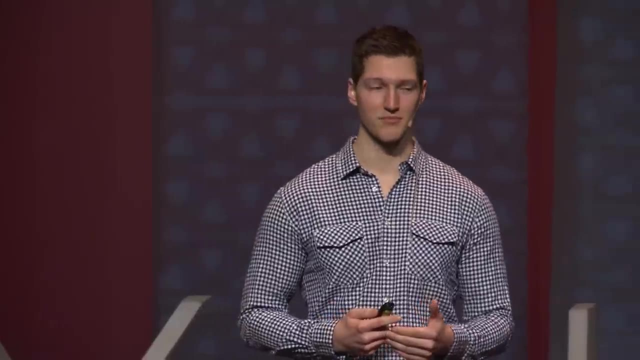 When you remove the barriers to your success- in my little brother's case, unhealthy food- and you pave the way barrier-free, the road to success becomes a much smoother ride. So set up your environment so that it works for you instead of against you. 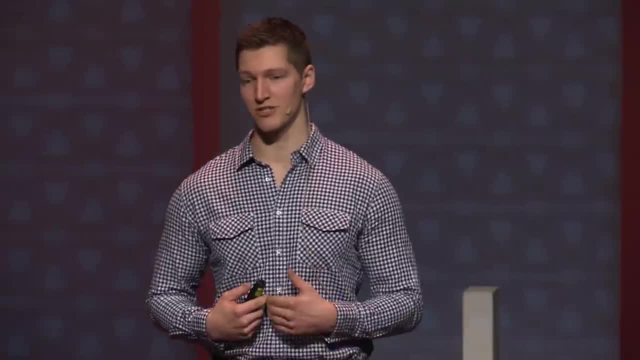 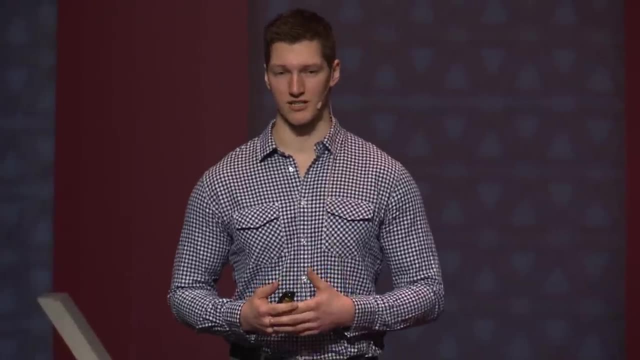 This works well for any goal. For my little brother, I was the environment. I made all of his food, gave him the right snacks and answered all of his questions. But what would that have looked like if I wasn't there? and how can you make this work for you? 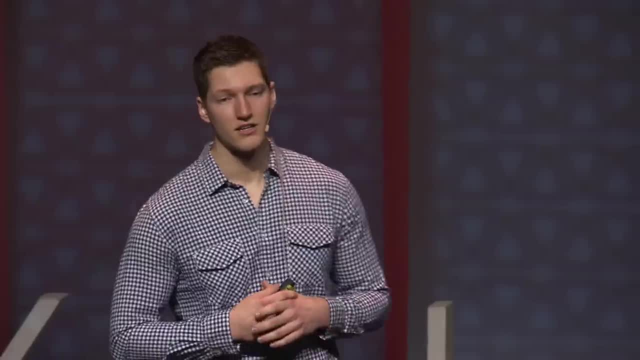 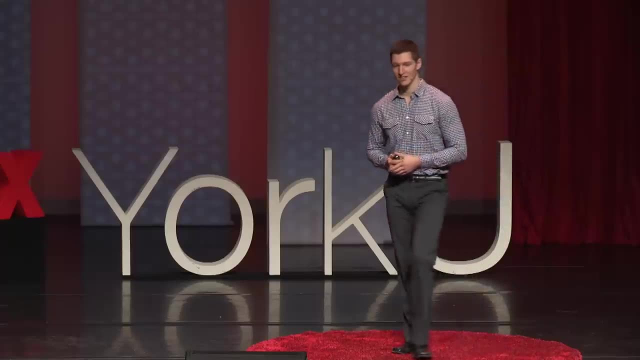 Well, to be successful you have to minimize the difficult decisions being made. Say, for example, you walk out into the lobby and on the left of those tables is delicious chocolate chip, cookies, squares and everything alike. On the right side is fresh fruit and vegetables. 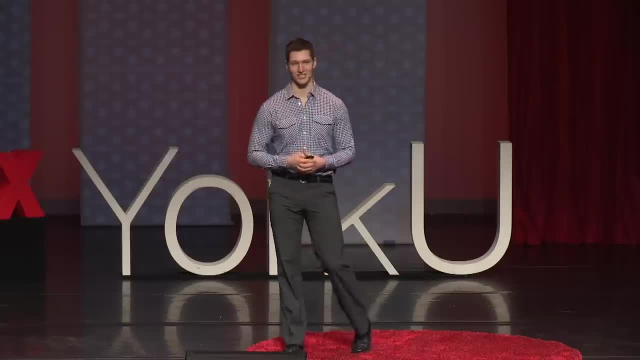 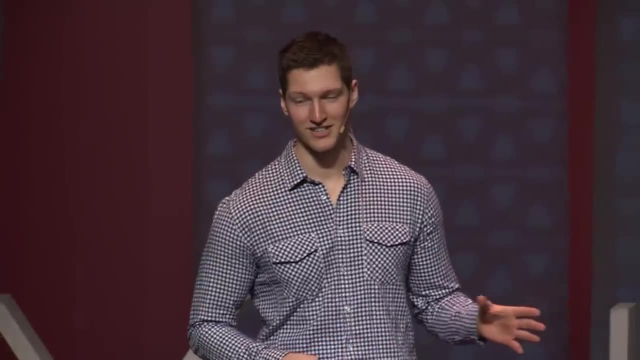 Vibrant colors, chopped up nicely. they're crunchy and juicy. Now you've been sitting in here for two hours so you're starving. You have a choice to make. Should you choose option A on the left, or should you choose the wholesome, nutritious? 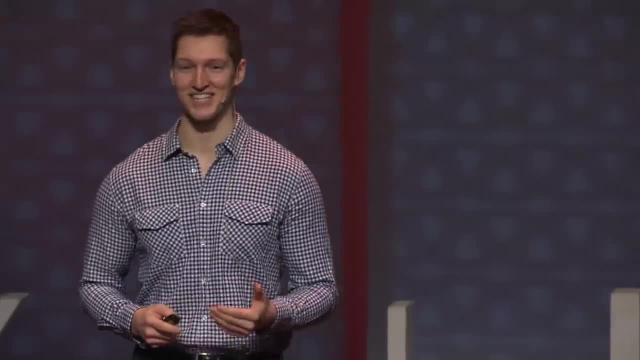 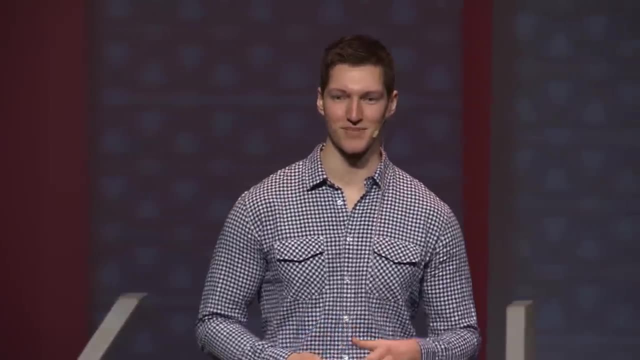 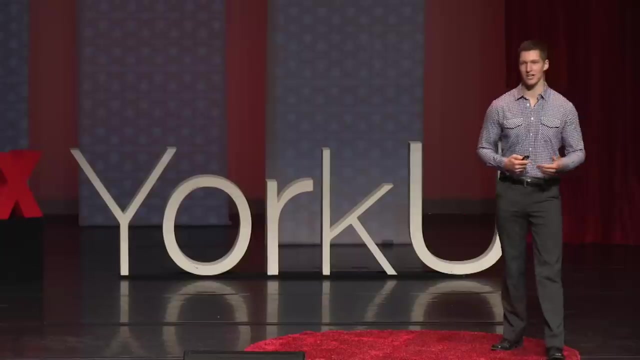 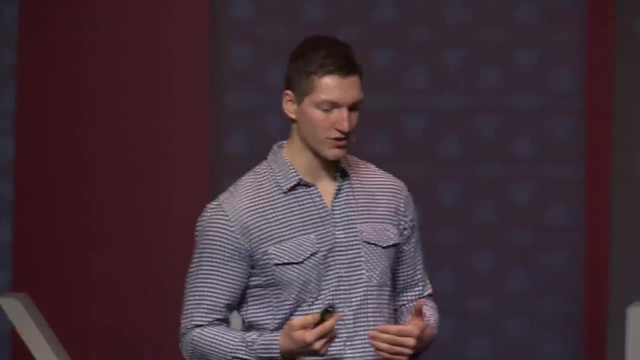 broccoli on the right Now. given this scenario, I think it would be very hard for most of us to resist the temptation of option A. Now, this is a real-life situation and it's one that happens all the time. It's very important because of that reason. 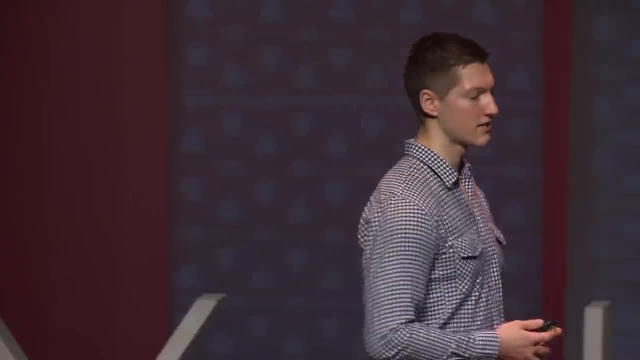 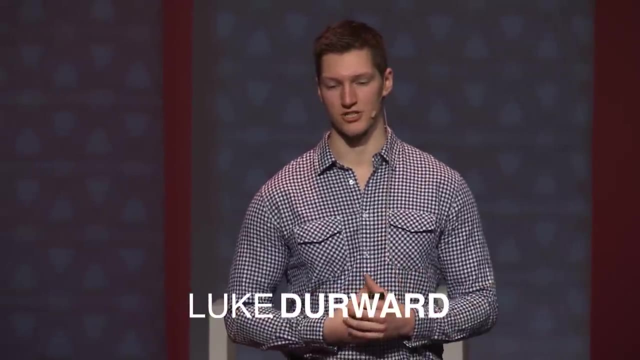 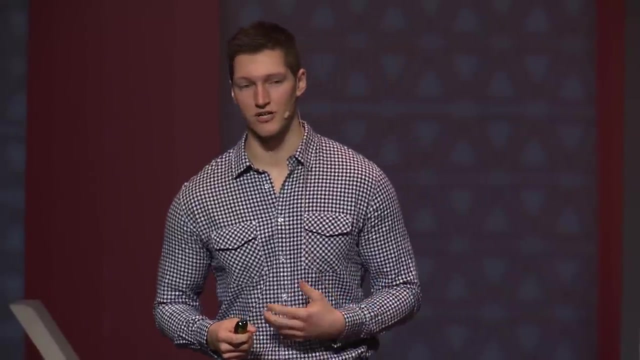 So when you remove the barriers to your success, it will just become a little bit easier for you to not have to make that hard decision in the first place. Here's how you can make this strategy work for yourself. Start off by finding out what your personal trigger foods are. and make a promise to not keep them in your house anymore, So that when the time comes, the decision has already been made for you. Now. that's not to say you can never have these foods again. If you really want one, you can always just go to the store and buy one.